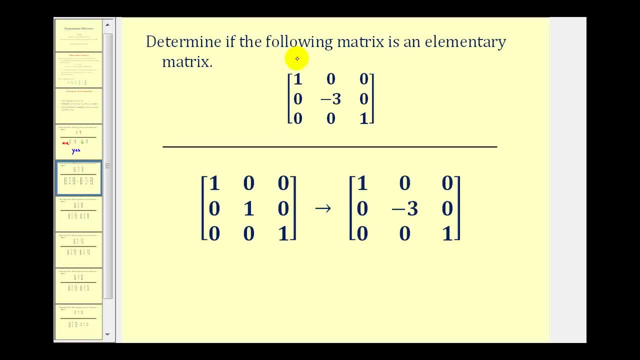 Let's look at several more examples. Again, we're given this matrix, so we want to start with a three by three identity matrix and see if we can obtain the given matrix by performing one row operation. Notice: the only change is this element here is negative three. 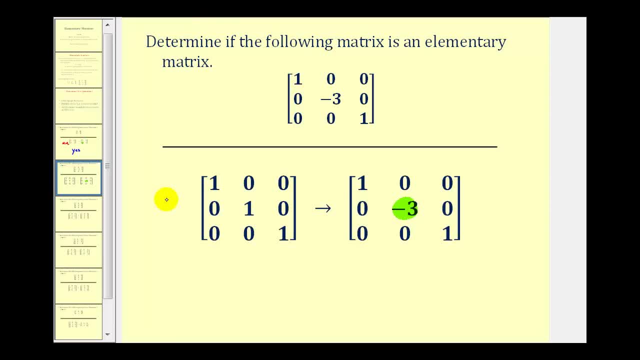 so if we were to replace row two with negative three times row two, notice how we would obtain the given matrix. and therefore, again, the answer is yes, this is an elementary matrix. Next, this is the given matrix. so we start with the three by three identity matrix. 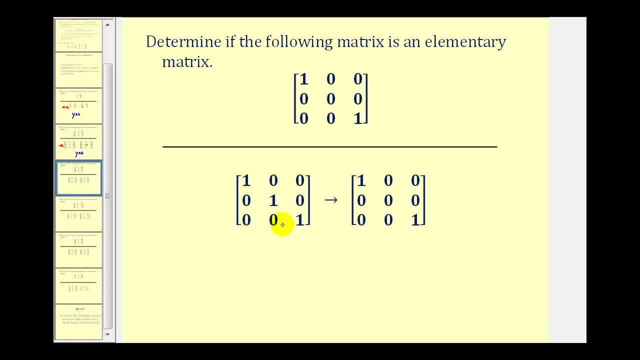 and see if we can obtain the given matrix by performing one row operation on the identity matrix. Again, notice: the only change is this: element here is zero. so we might be thinking we can just replace row two with zero times row two. but multiplying a row by zero is not an elementary row operation. 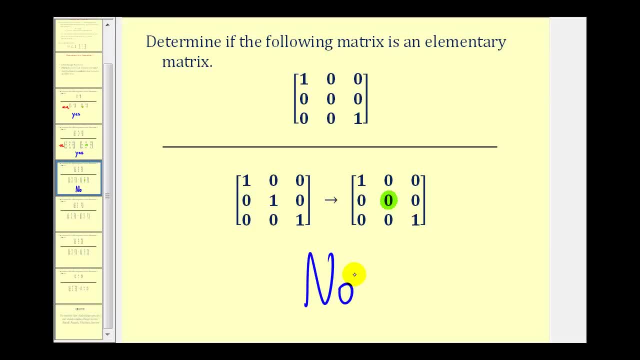 and therefore the answer is no. this is not an elementary matrix. Now we're given this three by three matrix Again, starting with the three by three identity matrix. we want to see if we can perform one row operation in this identity matrix to obtain the given matrix. 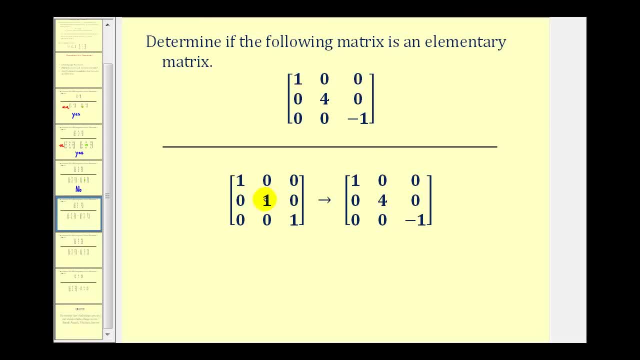 Well notice how this matrix here has been changed two ways. This one is now four and this one is now a negative one. So the only way to obtain the given matrix would be to replace row two with four times row two and to replace row three with negative one times row three. 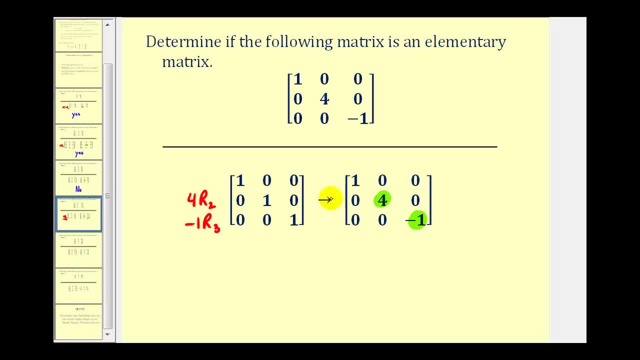 Well, this would be two elementary row operations, and for this to be an elementary matrix, we can only perform one row operation and therefore, again, the answer is no. this is not an elementary matrix. Let's look at two more examples. 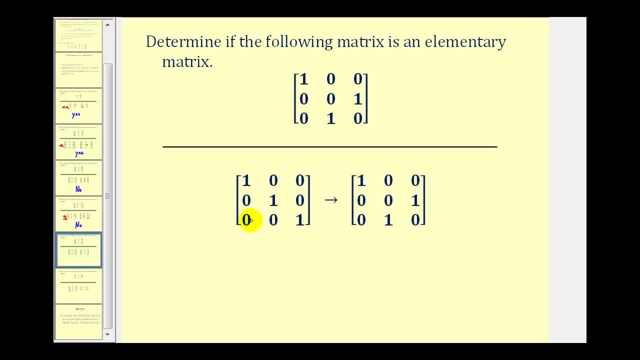 This is our given matrix. so we start with the three by three identity matrix and see if we can perform one row operation to obtain the given matrix. Well, notice, in the given matrix, or this matrix here, these two elements have changed and so have these.